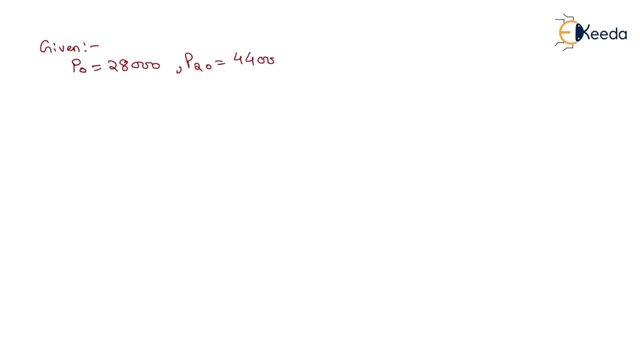 Now the population after 20 years is given as 44,000. So that will be the population after 20 years. Now we need to determine the increase in population per decade, that is x bar. Now, according to the arithmetic increase method, we know the formula of Pn equals to P0 plus nx bar. 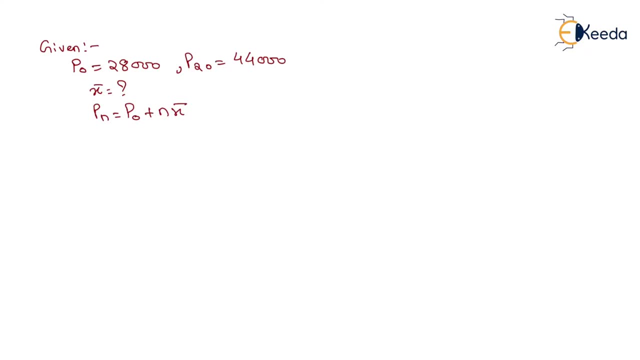 Here the Pn is given as 20.. P20 value is given as P0 plus nx bar, 44,000, and the P0 is given as 28,000.. And we need to determine the value of x bar and the n is given as 2.. 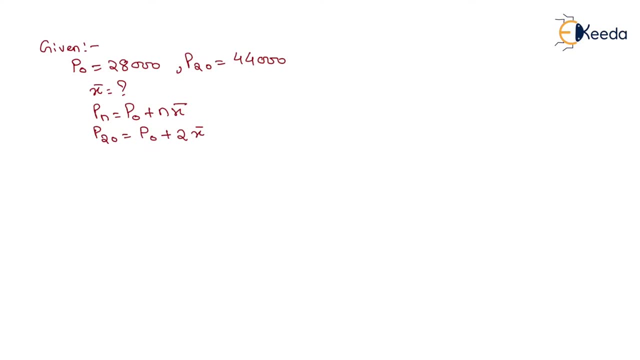 Why 2?? Because the difference in year is 20 year. So for the computation of number of decade we generally divide the number of years by the 10. That will be the number of decade. Now, from this formula we just put the value that is, 44,000 equals to 28,000. 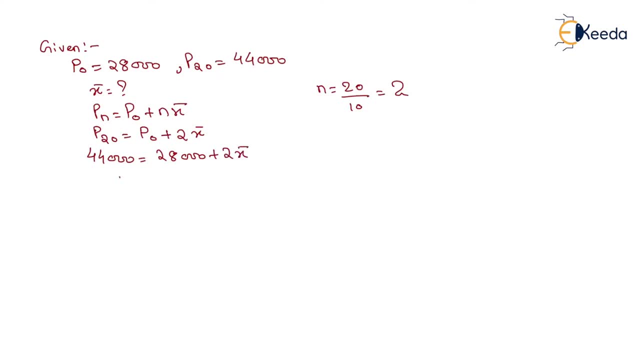 plus 2x bar. Now from this equation we will determine the value of x bar, which will be equals to 8,000.. Now that will be the value of population increase per decade. Now, another thing given in the equation is for the water consumption of 4,200 m3 per day. 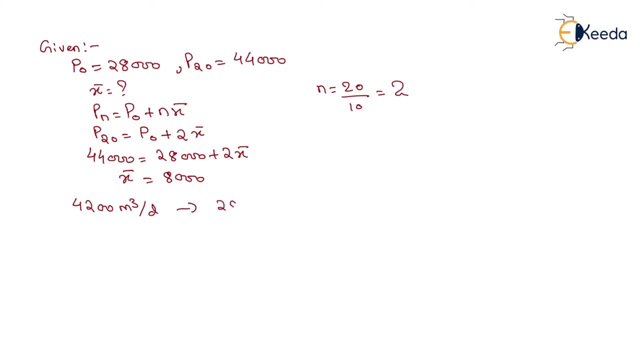 the population will be equals to 28,000.. Now we want to determine the population for the water consumption of 6,000 m3 per day. For 6,000 m3 per day consumption, what will be the population? Now we just take the values from here. 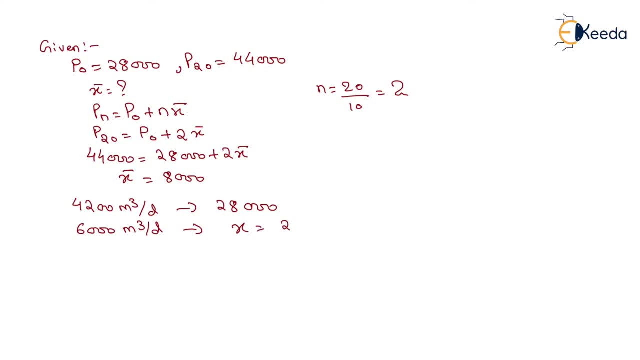 That will be equals to 28,000 into 6,000 divided by 4,200.. So the population comes out to be equals to 40,000 persons. It means that for 6,000 m3 per day consumption of water. 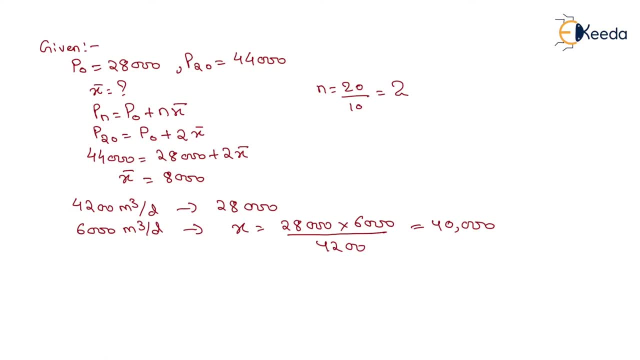 the population comes out to be 40,000.. Now we need to determine the number of years for which the plant will reach its design capacity. Now we have initial population, which is already given in the equation, which will be equals to 28,000.. 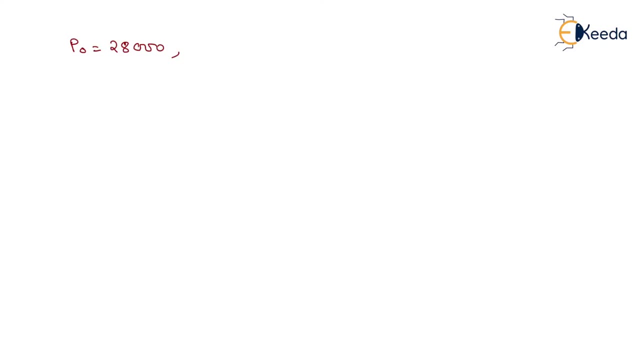 Now the population. when the plant will reach its water consumption of 6,000 m3 per day, its population is given as 40,000.. That will be the new population after N decade, that is 40,000.. Now we again use the formula that is: Pn equals to P0 plus Nx bar. 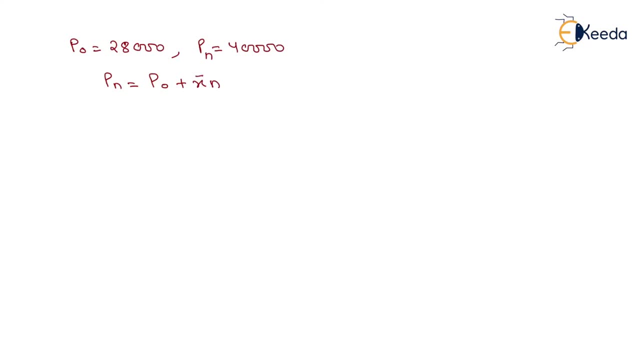 Now we have the value of Pn, which will be equals to 40,000.. We have the value of P0, which will be equals to 28,000.. We had already determined the value of x bar as 8,000.. And we need to determine from here the value of N. 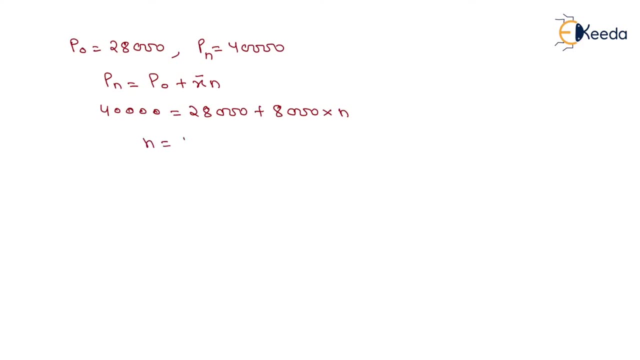 From this equation we will get the value of N equals to 1.5 decade. Now. if we want to convert this decade into year, then it will be equals to 15 years. Now for the water consumption of 6,000 m3 per day. 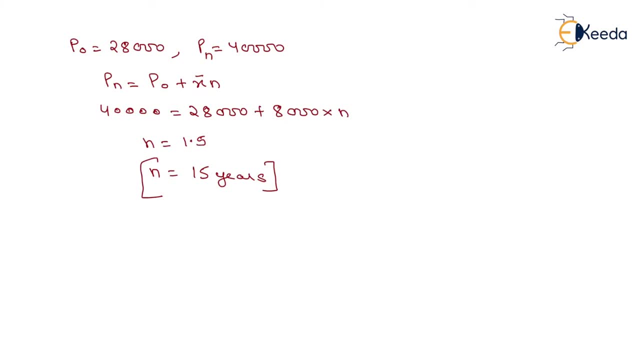 the number of year will be 15 years. It means that the number of year which will be coming in this question is equals to 15 years. That will be the solution of this question. Now we can move to the next question, That is: 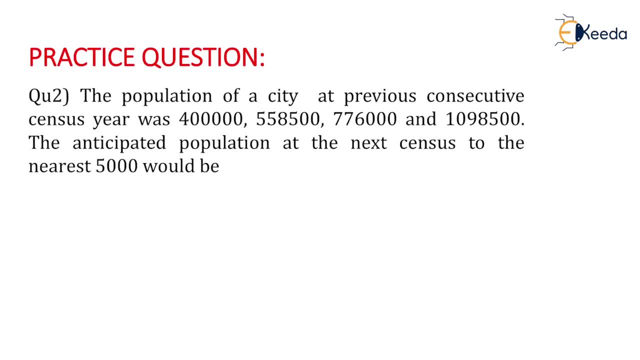 The population of a city at previous consecutive census year was 4,558,500, 7,76,000 and 10,98,500.. Now the anticipated population at the next census to the nearest 5,000 will be: Now in the question, method is not given. 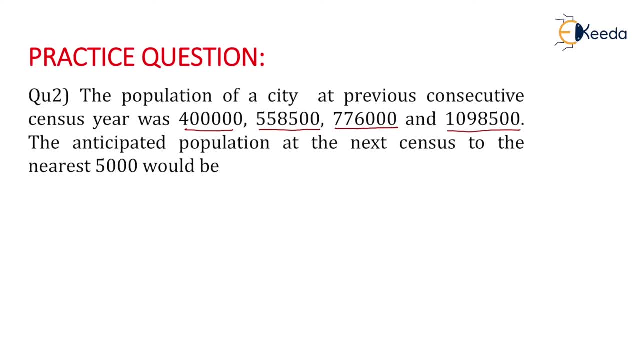 or precise method is not written in the question, And we know that if the method is not given in the question, then we have to use the incremental increase method. So we just make a table here In which the first one is the year. 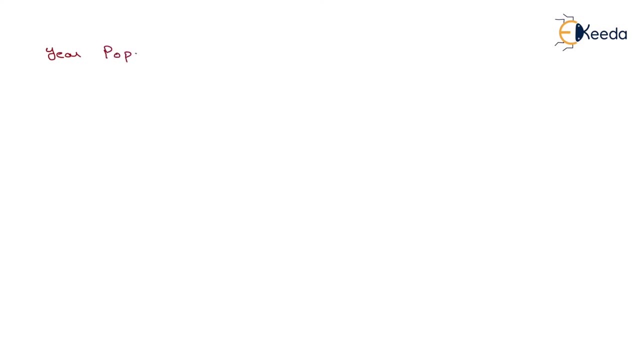 Second one is the population, which is given in the question. Now, the next will be the increase in population. Okay, Increase in population per decade. After increase in population per decade, we need to determine the incremental increase. Okay, Now, the year is given as equals to: 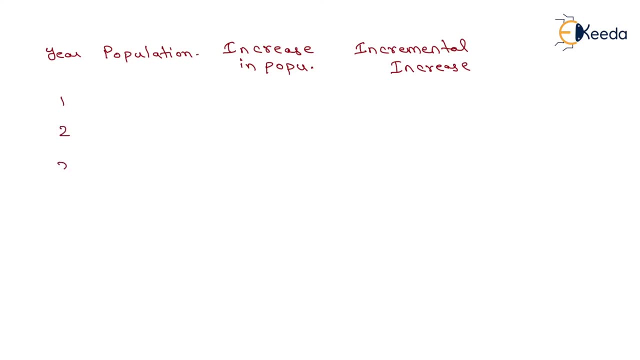 first year, second year, third year and fourth year. Now the first year population is given as 4 lakhs, So we just write here 4 into 10 to the power 5.. Okay, Now the next year population is given as 5,58,500. 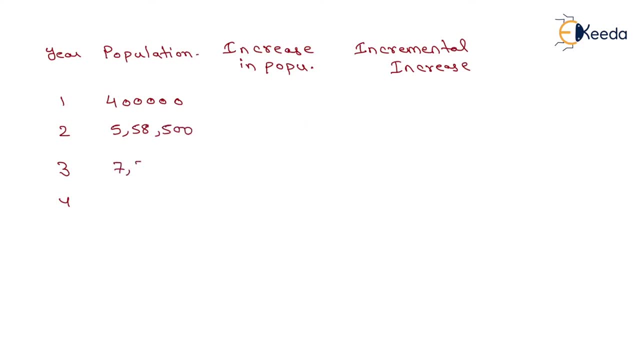 Okay, Now the next year population is given as 7,76,000.. Clear. And the last population which is given in the question is 10,98,500.. Now we need to find the increase in population per decade for which we need to subtract the value from this to this. 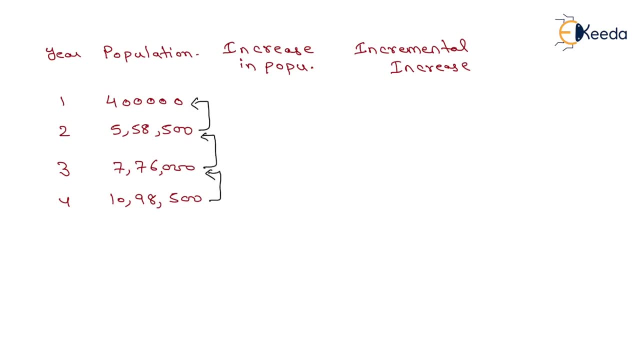 Now, from this to this, and from this to this. Now, when you subtract the value that is 5,58,500 and 4 lakhs, it will be coming out as 1,58,500. That will be the increase in population in first decade. 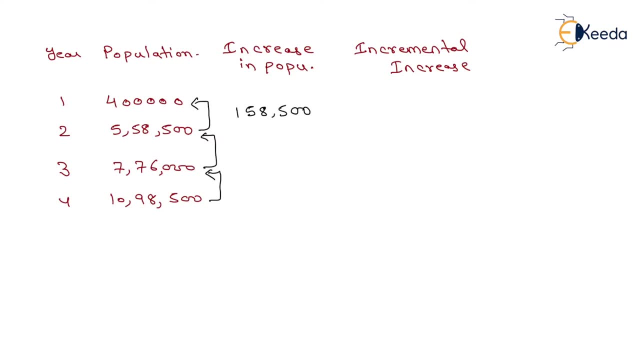 Okay, Now similarly, we can compute the increase in population. after second decade, It will be equals to 2,17,500.. Similarly, for the last decade, it will be equals to 3,22,500.. Now we need to find the incremental increase. 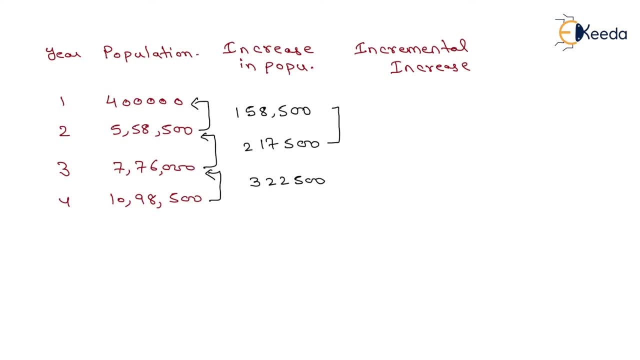 For incremental increase, we need to subtract the 1,58,500 from the 2,17,500.. So it will be equals to 59,000.. And similarly, when you subtract this value from this, you will get the answer as 10,05,000. 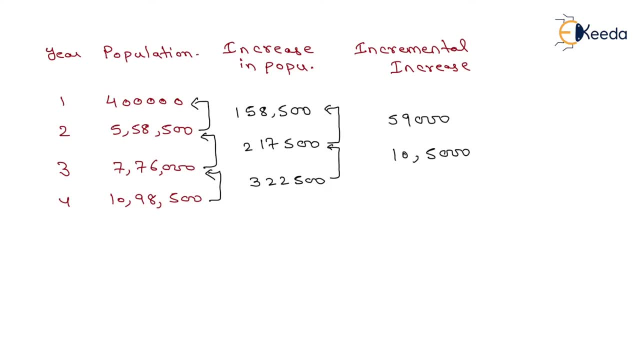 Okay, Clear. Now we need to find the x-bar and y-bar. For x-bar calculation, we need to add all this value and divide it by 3, because the number of decade is 3.. Okay, Now, if you add all this value and you divide all this value, 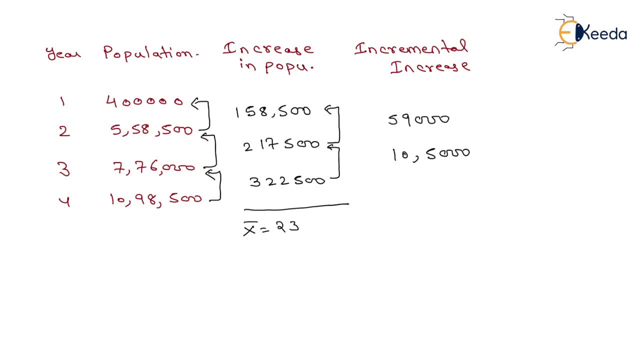 then the x-bar will be coming out. It will be equals to 2,32,833.33.. Similarly, if you add all this value and divide it by 2,, you will get the value as 82,000.. That will be the value of y-bar. 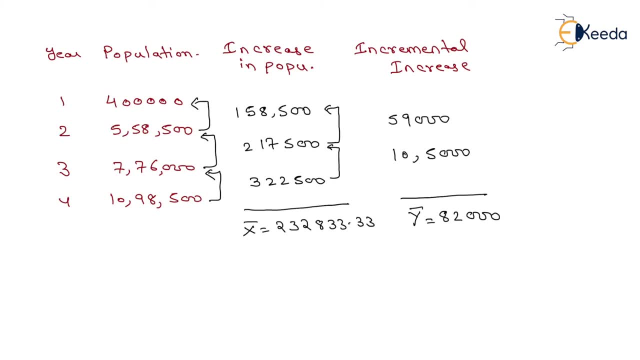 Now you have the value of x-bar and y-bar. Now you want to compute the population of fifth year. Now, if you want to compute the population of fifth year, what will be the value of n? It will be equals to equals to 1 year.